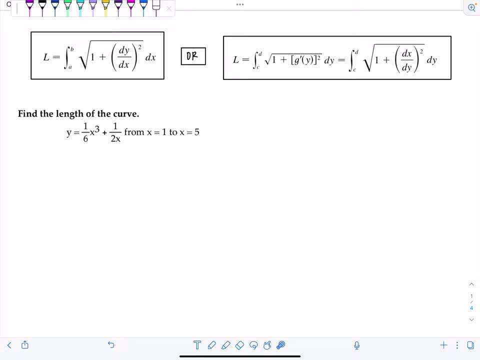 problem where there's this little factoring slick maneuver you have to do in order to be able to integrate And then, once you know it, you'll be a pro anytime. you see it, I like to get everything ready to integrate before I write out my full integral, So I like to take the 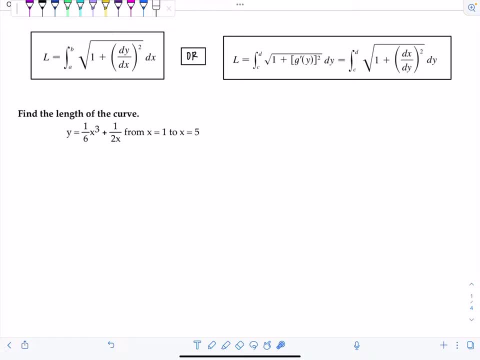 derivative square. it add one, clean it up as much as possible and then write out my full integral. Okay, And before I take the derivative, I'm going to rewrite my function y, So it's a little more obvious how to differentiate. So I'm going to write this as one half x to the negative. 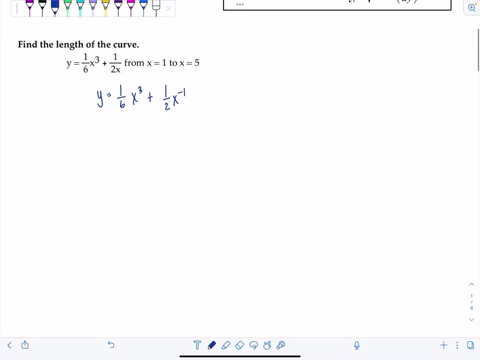 first. That's it. Okay, now it's derivative time. So, dy dx, I'll go slowly for now, just as you're warming up. 1 sixth, I'm going to bring the 3 down. Now I have x squared plus one half times negative. 1 times x to the negative second. Yes, Oh good, So now we're. 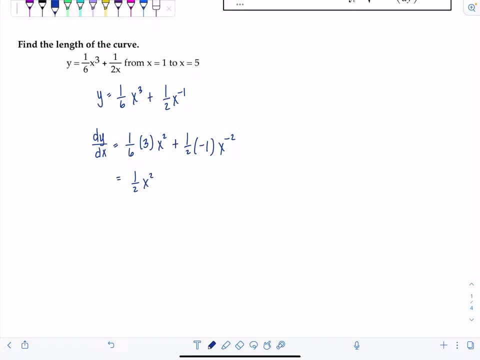 left with one half x squared minus 1 over 2x squared. Okay, so that's our derivative. That's dy dx. That's not what we integrate. What we integrate is the square root of 1 plus dy dx squared. So let's see what happens when we 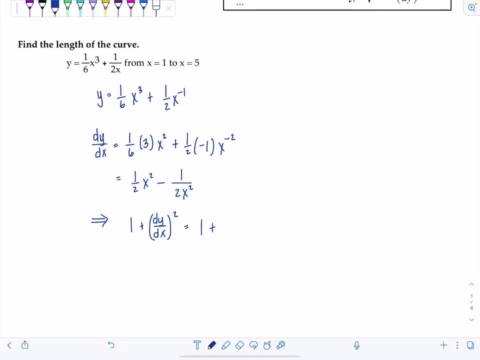 take it a step further. This is going to be 1 plus. I'm squaring one half x squared minus 1 over 2x squared, Like that. Okay, so let's see, here We're going to have 1 plus, remember. 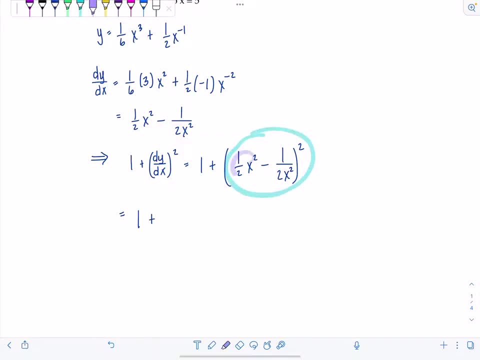 when you square a binomial like this, you square the first term, So that would give us 1 fourth x to the fourth Minus. keep the sign the same. Then you multiply these two terms by each other and double it. So I'll do that off to the side One half x squared times 1 over 2x squared. 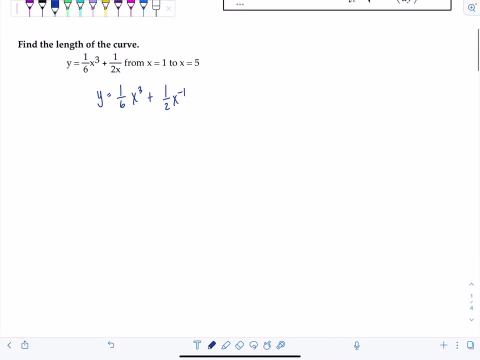 first. That's it. Okay, now it's derivative time. So, dy dx, I'll go slowly for now, just as you're warming up. One sixth: I'm going to bring the three down. Now I have x squared plus one half times negative. one times x to the negative second. Yes, Oh good. 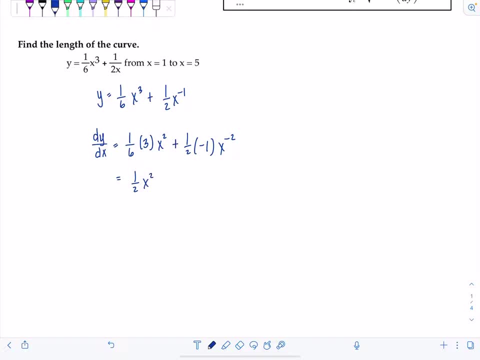 So now we're left with one half x squared minus one over two x squared. Okay, so that's our derivative. That's dy dx. That's not what we integrate. What we integrate is the square root of one plus dy dx squared. So let's see what happens. 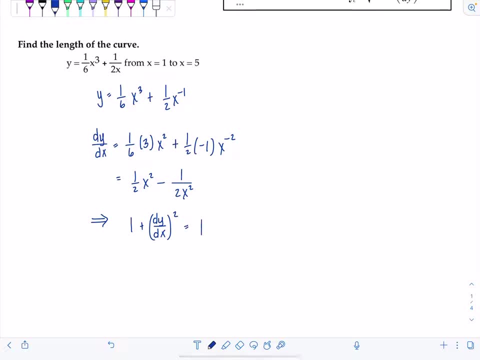 when we take it a step further, This is going to be one plus. I'm squaring one half x squared minus one over two x squared, Like that. Okay, So let's see, here we're going to have one plus. remember when you. 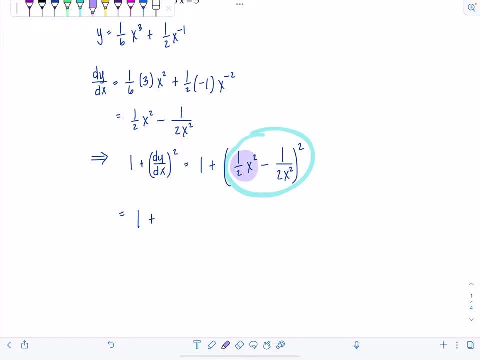 square a binomial like this: you square the first term, So that would give us one fourth x to the fourth minus. keep the sign the same. Then you multiply these two terms by each other and double it. So I'll do that off to the side. One half x squared times one over two x squared. What happens? 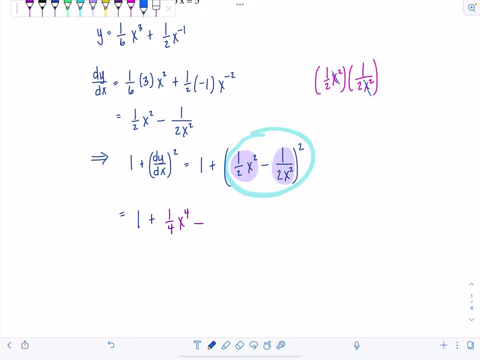 Well, the x squareds cancel, Boop, boop And I'm just left with one fourth. But what's my middle term? Two times that, Yes, Good. Plus, then we square the last term, So that would be one over four x squared. 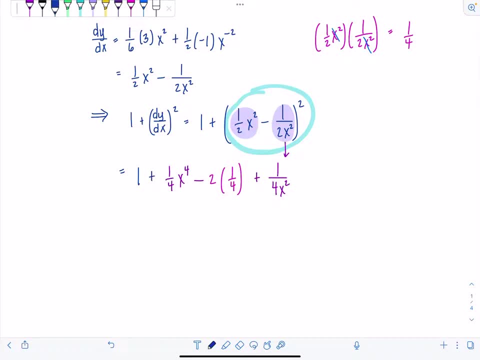 Okay. So let's see what's going on here. I've got one plus one fourth x to the fourth, minus one over two x squared. Okay. So let's see what's going on here. I've got one plus one fourth x to the fourth, minus one over two x squared. 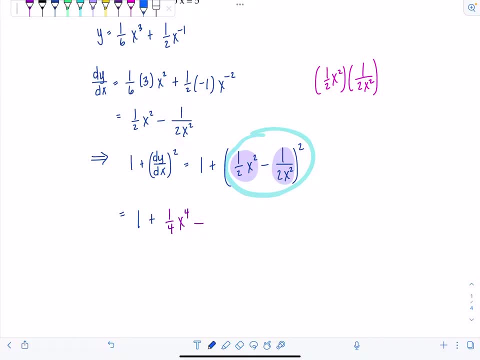 What happens? Well, the x squareds cancel, Boop, boop And I'm just left with 1 fourth. But what's my middle term? 2 times that, Yes, Good Plus. then we square the last term, So that would be 1 over 4x squared. 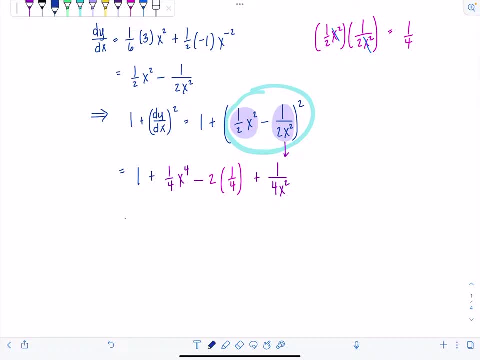 Okay. so let's see what's going on here. I've got 1 plus 1 fourth x to the fourth, minus a half plus 1 over 4x squared, And this will, if you're given a problem in this little form, it'll always work out so that you have a negative one half in the middle, And then you 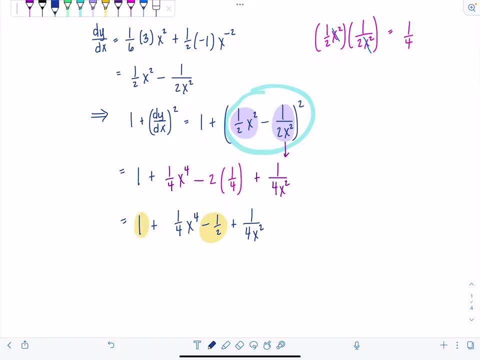 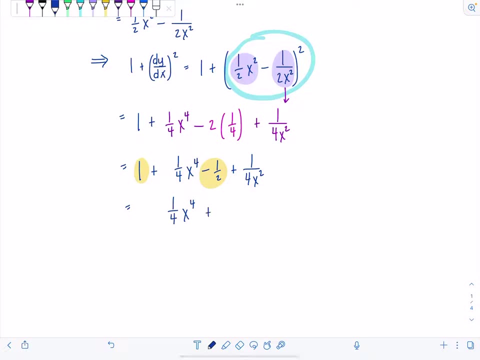 can combine that with the 1 and you have a positive one half, And I'm actually going to put the positive one half in the middle, You'll see why. So we've got 1 fourth x to the fourth plus one half plus 1 over 4x squared. 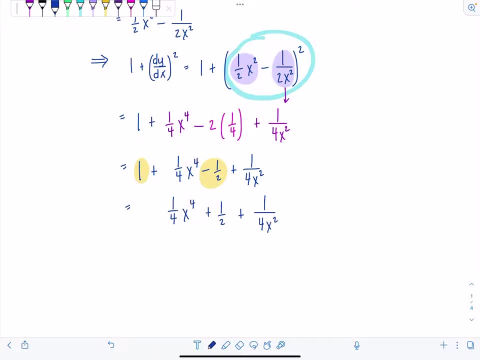 Now. I'm not going to write out my integral just yet. Remember, we're going to have to integrate the square root of this And I'm not happy with how it's looking right now. However, there's a trick. You need to recognize that this is a perfect square trinomial and it can be factored. 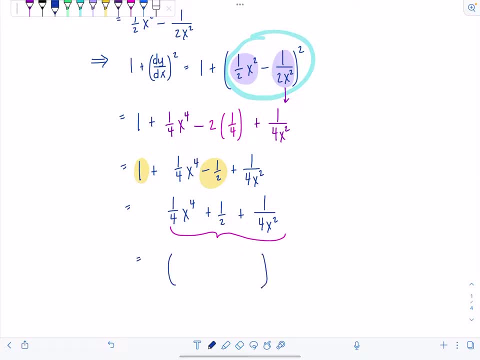 How You must be wondering. Well, I want you to take a peek up ahead above. Remember, when we multiplied out the derivative, What did we get? What did we get? Let me erase some of the highlighting so you can see what happened. When I multiplied it out, I had 1 fourth x to the fourth, minus a half plus. 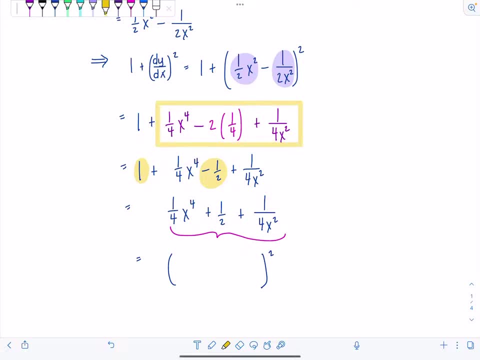 1 over 4x squared, And that's nearly identical to the three terms that we have here. What's the only difference? The only difference is that, instead of a negative one half, I now have a positive one half. What that means is it's going to factor just like dy dx, except I'll have addition between. 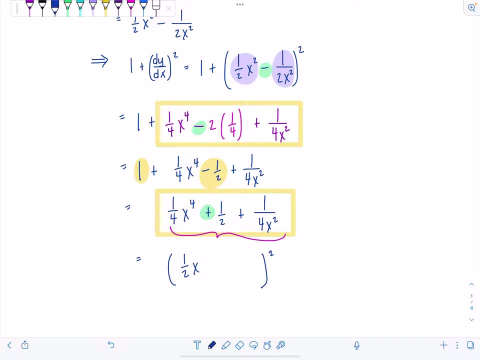 the two terms. So this is going to be one half x squared plus 1 over 2x squared. Take a second and think about it, And if you're thinking to yourself, oh my goodness, I would have never noticed that in a million years, That's okay, I'm telling you now. So next: 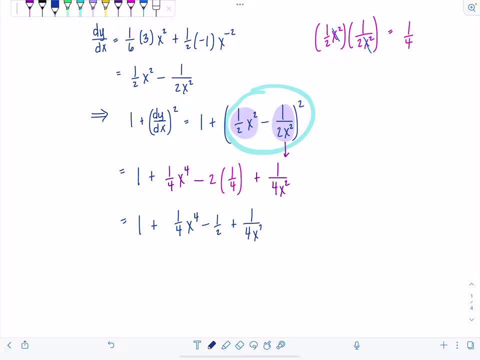 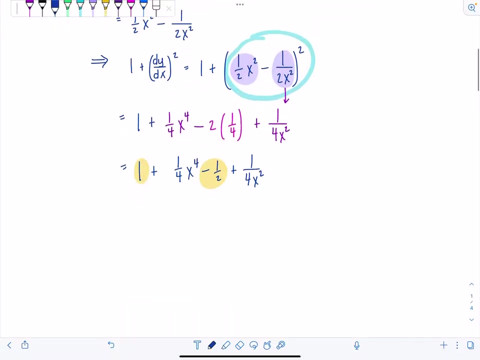 Minus a half, plus one over four x squared. And this will, if you're given a problem in this little form, it'll always work out so that you have a negative one half in the middle And then you can combine that with the one And you have a positive one half, And I'm actually going to put the positive one half in the middle, You'll see why. So we've got one fourth x to the fourth, plus one half plus one over four x squared. 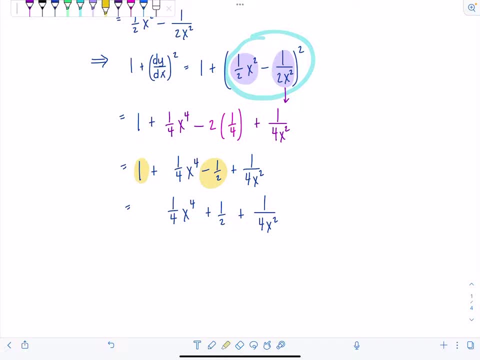 Now. I'm not going to write out my integral just yet. Remember, we're going to have to integrate the square root of this And I'm not happy with how it's looking right now. However, there's a trick. You need to recognize that this is a perfect square trinomial And it can be factored How You must be wondering. Well, I want you to take a peek up ahead above. Remember, when we multiplied out the derivative. 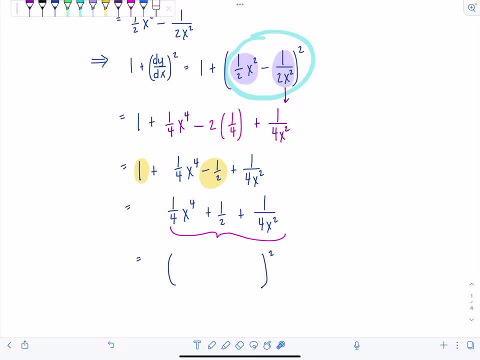 What did we Get? What did we get? Let me erase some of the highlighting so you can see what happened. When I multiplied it out, I had one fourth x to the fourth minus a half, plus one over four x squared, And that's nearly identical to the three terms that we have here. What's the only difference? The only difference is that instead of a negative one half, I now have a positive one half. So what that means is 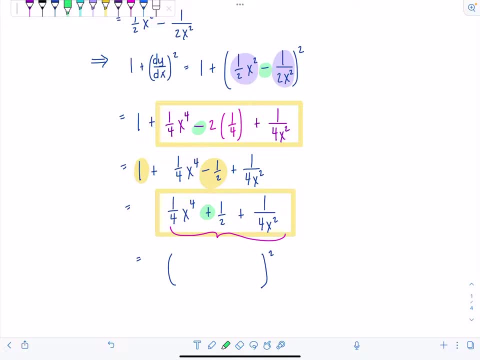 it's going to factor just like dy, dx, except I'll have addition between the two terms. So this is going to be one half x squared plus one over two x squared. Take a second and think about it. And if you're thinking to yourself, oh my goodness, I would have never noticed that in a million years, That's okay, I'm telling you now. So next time you see it you'll notice it. That's it. You know, don't feel badly. There are some people who don't need to be told these little hints. Good for them. 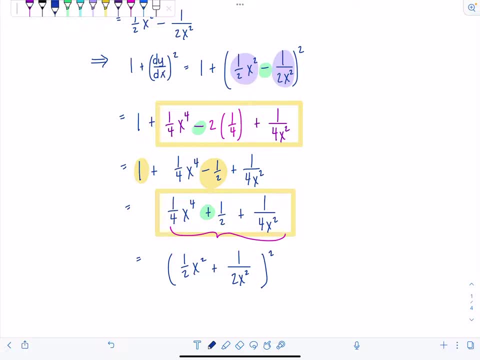 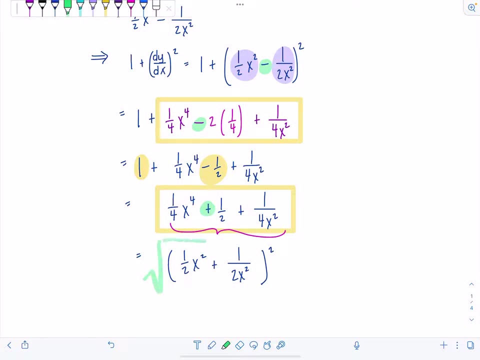 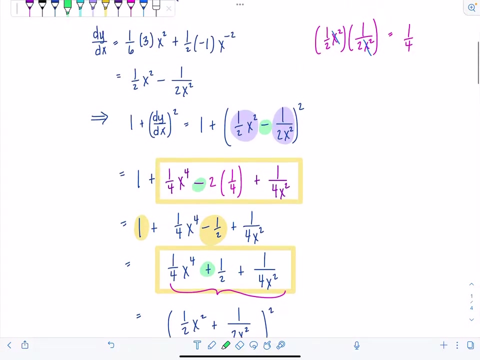 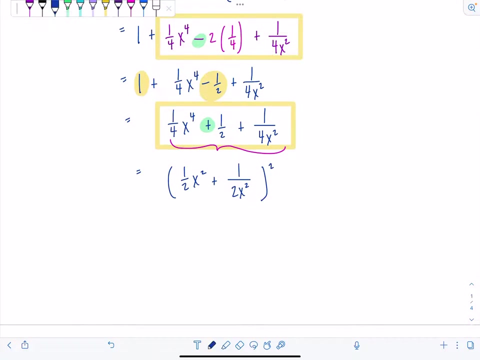 You can just keep practicing and you'll do it effortlessly as well. Now I'm really thrilled to integrate this, because if I have a big radical sign right, then it'll just cancel with the squared. my exponent: So great. We're ready to set up our integral. Limits of integration are one to five. So here we go. So arc length is going to be definite integral from one to five. I have square, one to five. 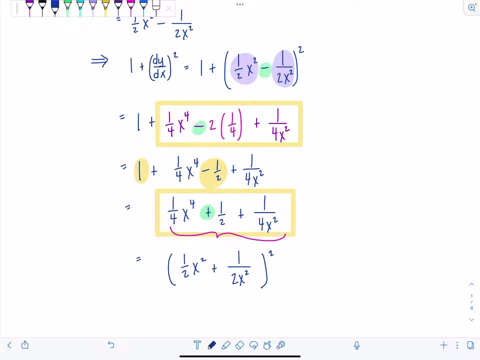 time you see it, you'll notice it. That's it, You know. don't feel badly. There are some people who don't need to be told these little hints. Good for them. But otherwise you can just keep practicing and you'll do it effortlessly as well. Now. 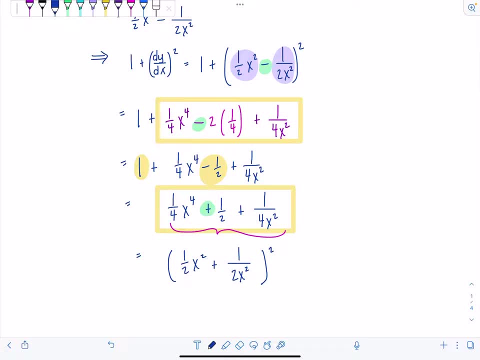 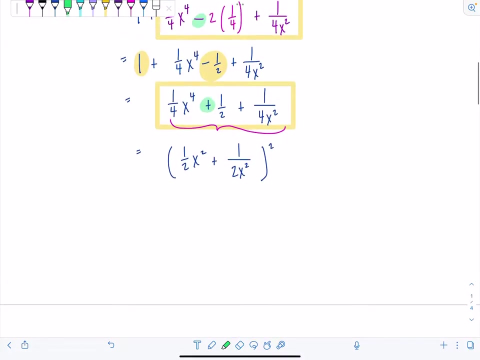 I'm really thrilled to integrate this, because if I have a big radical sign right then it'll just cancel with the squared. my exponent: So great, We're ready to set up. our integral Limits of integration are 1 to 5.. So here we go. So arc length is going to be definite. 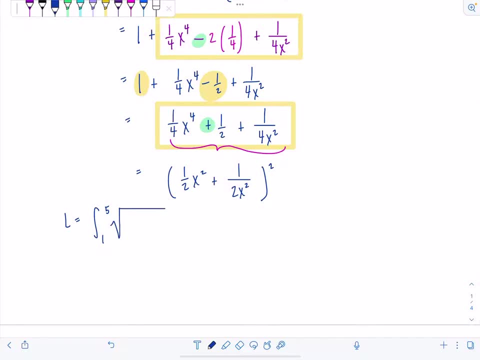 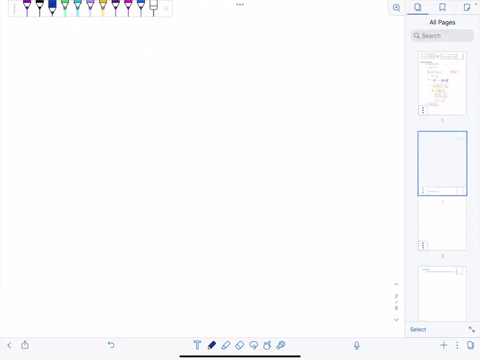 integral from 1 to 5.. We have square root of one half x squared plus 1 over 2x squared squared dx. Let me add a page because we're running out of space. Okay, And then from here I can just get rid. 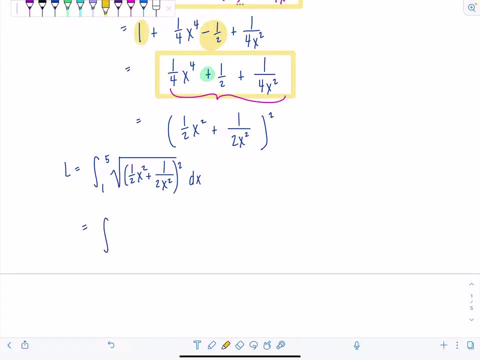 of the radical sign and cancel out the exponent here. These two undo each other. So we have definite integral from 1 to 5.. 12, 18, five- well, you know, technically it's absolute value of everything inside, but on one to five everything's positive. so I'm not worried. okay, and then let's see, we've got one half x squared. 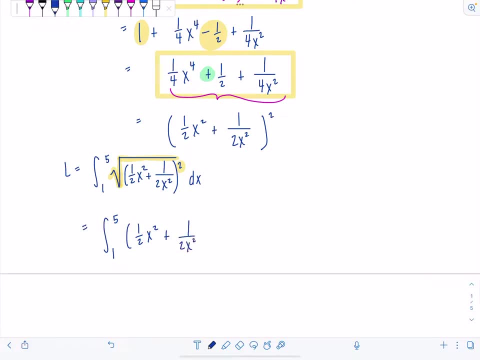 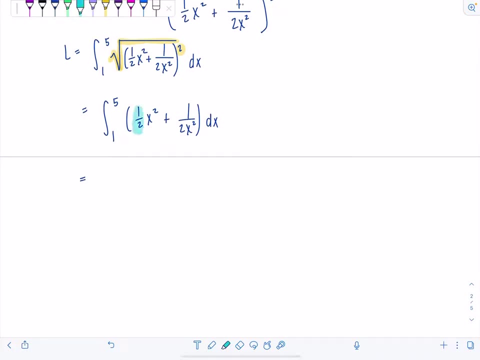 plus one over two x squared dx. do you know what I'm gonna do? I'm gonna take out a one half. mm-hmm, can't I do that? take out a one half from the whole thing, it'll make life nicer. one half, definite integral from one to five, and then now I have x squared plus. I'm gonna write: 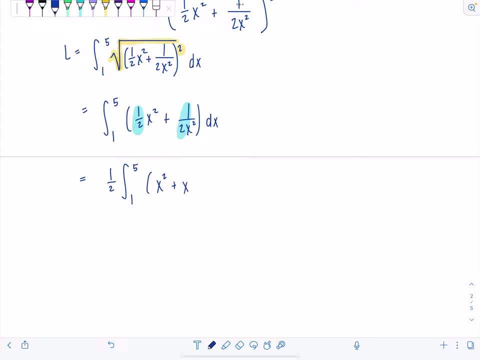 this as: x to the negative second. okay, that way I'm ready to integrate dx. so we've got one half times. uh, anti-derivative of, excuse me, x squared is one third of x squared, x cubed, x to the negative second. add one divide by the new exponent, so it would be negative. x to 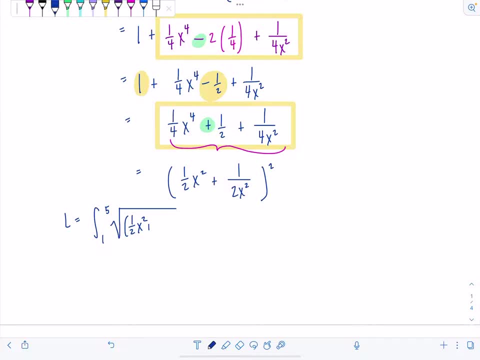 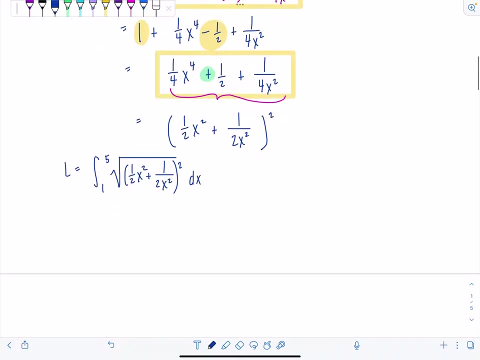 I have square root of one half x squared plus one over two x squared squared dx. Let me add a page because we're running out of space, Okay, And then from here I can just get rid of the radical sign and cancel out the exponent here. These two undo each other. So we have definite integral from one to five. 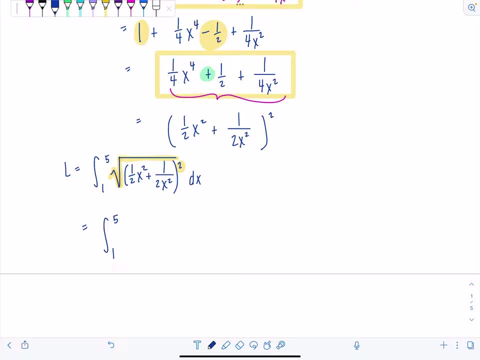 Well, you know, technically it's absolute value of everything inside, but on one to five everything's positive. So I'm not worried, Okay. And then let's see, We've got one half x squared plus one over two x squared dx. Do you know what I'm going to do? I'm going to take out a one half, Can't I do that? Take out a one half from the whole thing. It'll make life nicer. 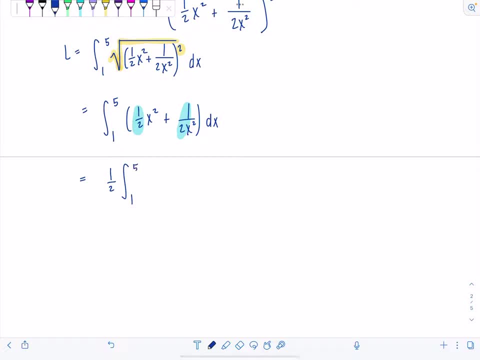 Okay, One half definite integral from one to five. And then now I have x squared plus. I'm going to write this as: x to the negative second. Okay, That way I'm ready to integrate dx. So we've got one half times antiderivative of. excuse me, x squared is one third, x cubed, X to the negative second. Add one Divide by the new exponent, So it would be one half. 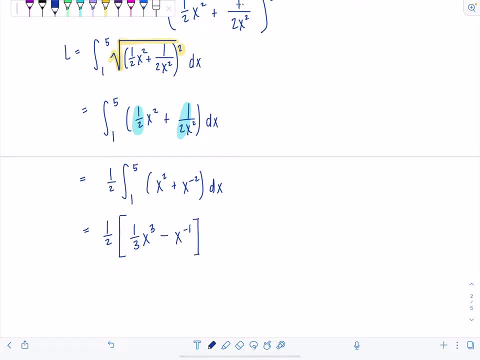 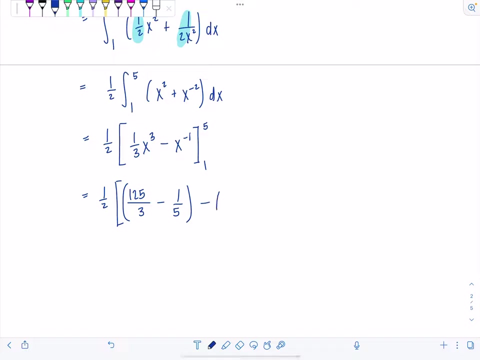 It would be negative. x to the negative first. I'm evaluating this from one to five. So let's see We're going to have one half times one third times five cubed, So that's 125 over three minus five. to the negative first is one fifth. That's the upper limit, minus one third minus one. 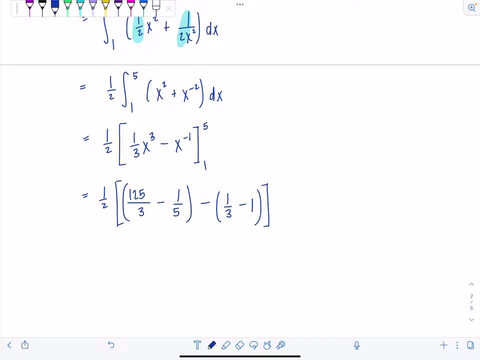 Okay, And then from there, common denominator is 15.. So here we go. We've got one half times, So 125 times five. Let's see, I'm just confirming 625 minus three If I multiply this guy by three. 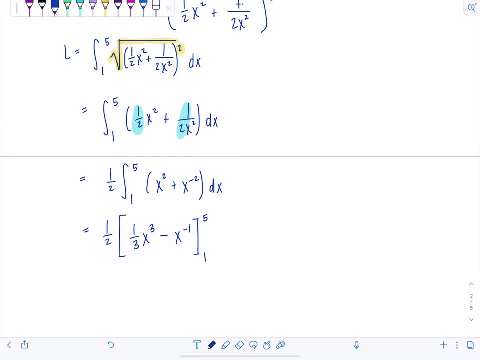 the negative first. I'm evaluating this from one to five. so let's see we're gonna have one half times one, third times five cubed, so that's 125 over three minus five. to the negative first is one-fifth, that's the upper limit minus. 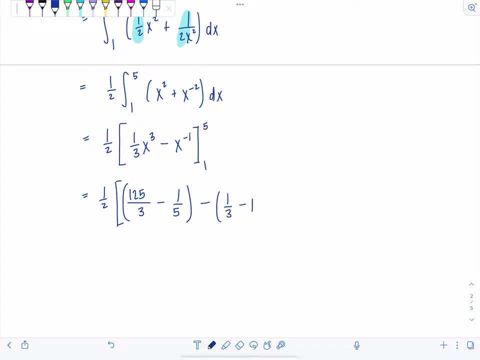 one-third minus one, okay, and then from there, common denominator is 15, mm-hmm. so here we go. we've got one half times, so 125 times five. let's see I just confirming 625 minus three if I multiply this guy by three, yes, by five, by five, and this by 15. so let's see I. 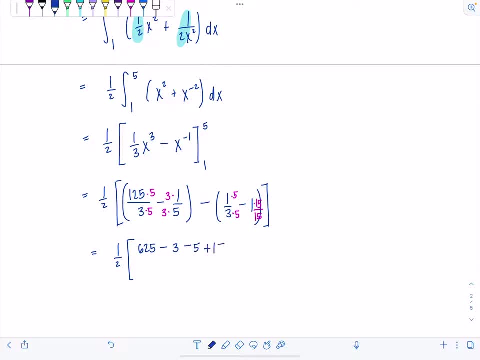 already got the minus three, then minus five plus 15 over 15. so we've got 625 minus eight plus 15, 632 over 15, and I've got that 1 half in the front so I can cancel 1 half with 632, and 632 is going to become 316. so our final answer: 316 over 15 units. 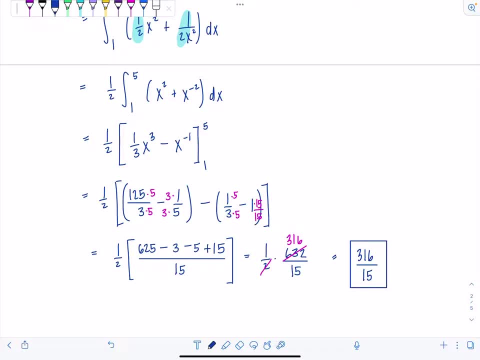 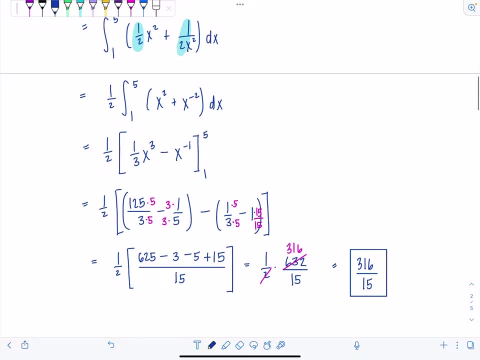 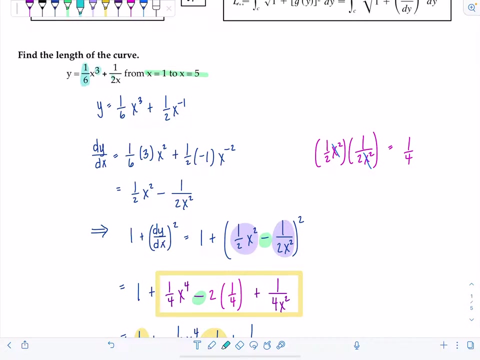 okay, one dimensional answer because it's arc length. all right, you'll see this same sort of integral arc length problem repeatedly. the only thing that will change are, like the mix of coefficients and exponents here, but you'll be doing the same sort of factoring maneuver. 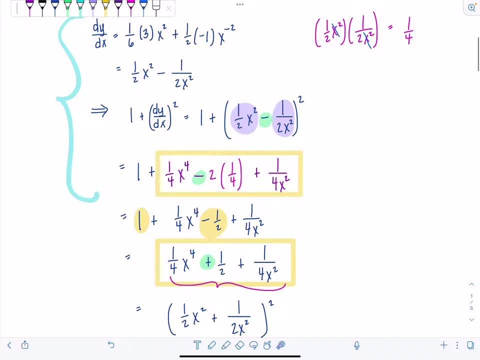 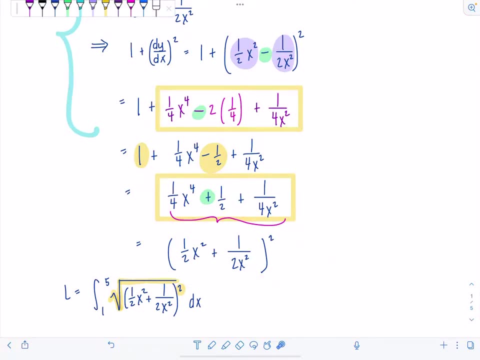 where you have that negative 1 half right here, that after you add it to the one, you're left with a positive 1 half, and then you just refactor it and you're left with a negative 1 half. it's in every book, it's in every homework section. it's nothing new, so just remind yourself that. so 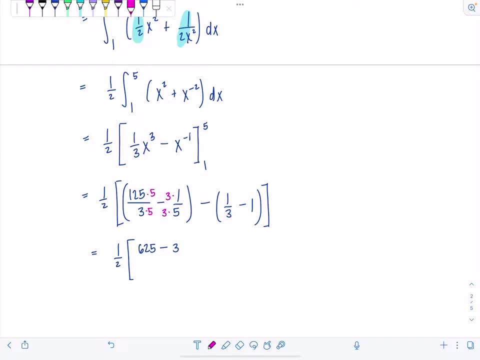 Yes, By five, By five, And this by 15.. So let's see, I already got the minus three, Then minus five plus 15 over 15.. So we've got 625 minus eight plus 15.. 632 over 15.. 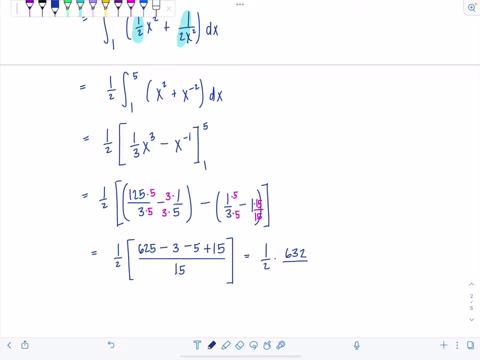 And I've got that one half in the front So I can cancel one half with 632.. And 632 is going to become 316.. So our final answer: 316 over 15 units. Okay, One dimensional answer because it's arc length. 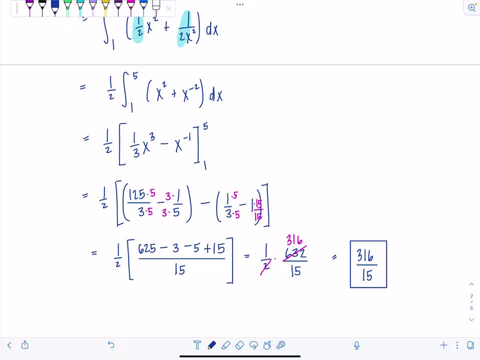 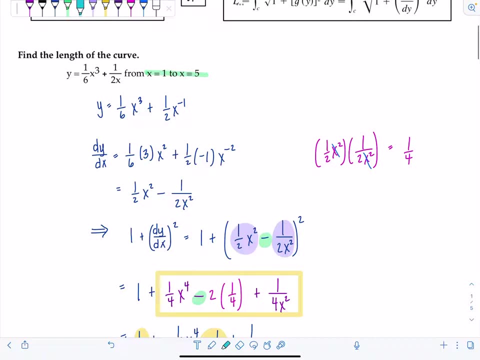 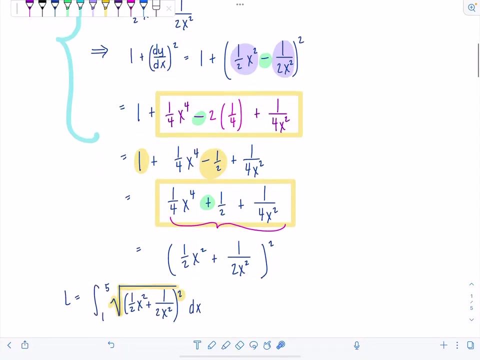 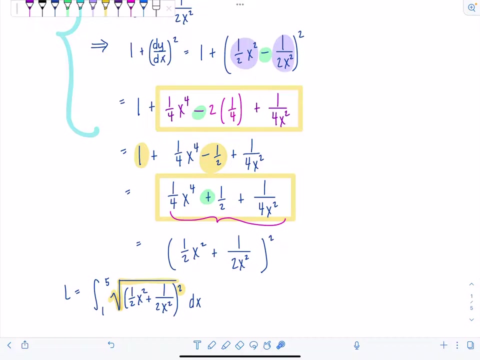 All right, You'll see this same sort of integral arc length problem repeated. The only thing that will change are, like, the mix of coefficients and exponents here. But you'll be doing the same sort of factoring maneuver where you have that negative one half right here, that after you add it to the one, you're left with a positive one half, And then you just refactor. It's in every book, It's in every homework section. It's nothing new. So just remind yourself that so you don't get so freaked out. 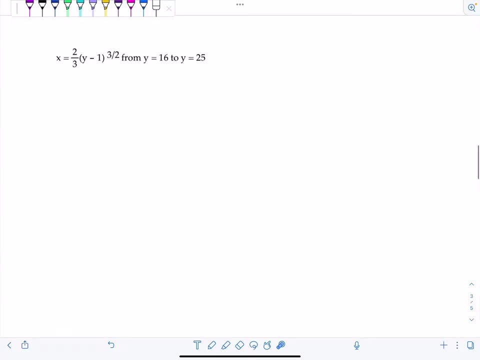 Okay, I got another one for you. this time Let's integrate. Let's integrate with respect to y. So x equals two thirds times y minus one to the three halves, And we're going to find the arc length from y equals 16 to 25.. So you can already see it's set up for us. X is a function of y, The limits are in terms of y. Why would you not want to integrate with respect to y? 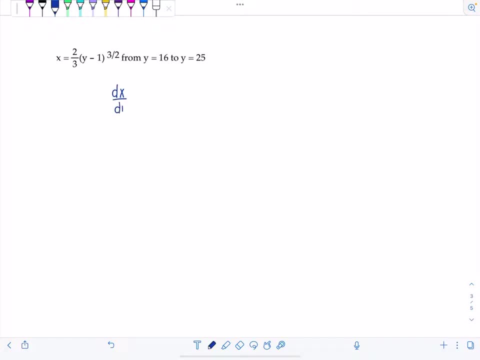 So let's find the derivative dx dy. Somebody loves this because look, you have two thirds times three halves times Y minus one now to the one half, And then derivative of y minus one is just one. So two thirds, three halves, cancel. I'm just left with y minus one to the one half. That's not what I'm integrating, though Remember I have one plus dx dy squared, So that's going to be one plus y minus one to the one half squared. 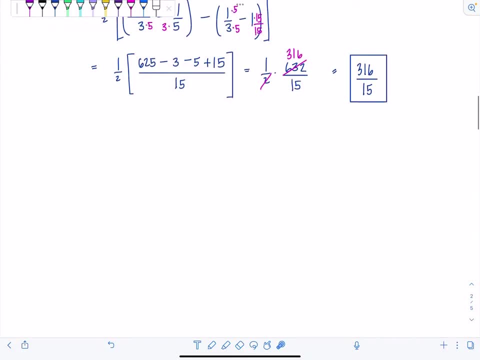 you don't get so freaked out. okay, I got another one for you. this time let's integrate with respect to y. so x equals 2 thirds times y minus 1 to the 3 halves and we're going to find the arc length from y equals 16 to 25. so you can already see it's set up for us. x is a function of y, the limits are: 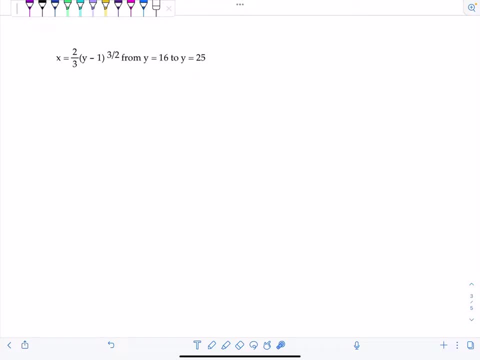 in terms of y, why would you not want to integrate with respect to y, you? so let's find the derivative dx dy. somebody loves us because, look, you have two thirds times, three halves times y minus 1. now to the one half, and then derivative of y minus 1 is just 1. so two thirds, three halves, cancel, I'm just left. 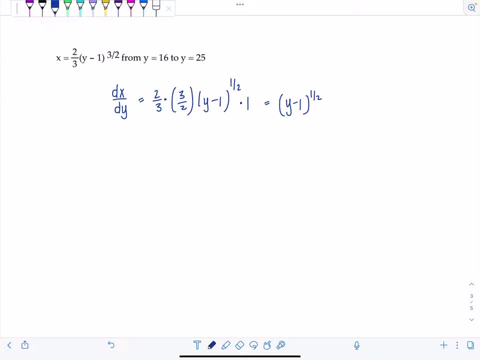 with y minus 1 to the one half. that's not what I'm integrating, though. remember I have 1 plus 2key xty squared, so that's going to be 1 plus y minus 1 to the one half squared. oh so lovely. this is 1 plus y minus 1, which is just why this is what. 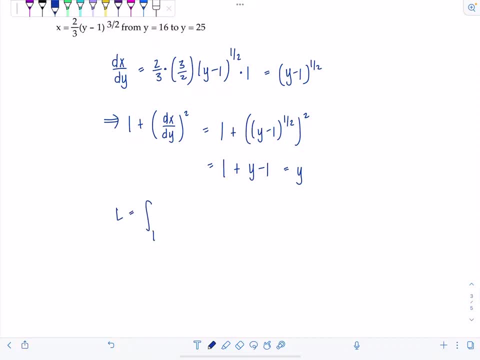 dreams are made of. so arc length is gonna be definite integral from 16 to 25, square root of y, dy. so 2 darüber 107岁, 15 x15电의 xd y pants yweh. that's y, y, h, o, y, o, y to the one half. If I integrate, I'm going to add one to the exponent, So it'll be y to the. 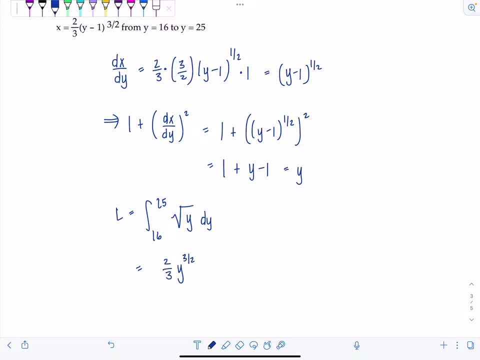 three halves, divide by the new exponent and then evaluate this from 16 to 25.. Okay, so we've got two thirds times 25 to the three halves, minus 16 to the three halves. We don't need a calculator for this, Oh no, no, no. So 25 to the three halves. 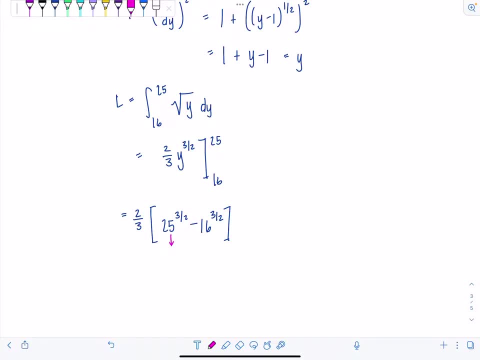 you take the square root of 25, and then cube it. So five cubed is 125.. Same thing 16 to the three halves. you take the square root because you have a two in the denominator four, and then cube it, that's 64.. 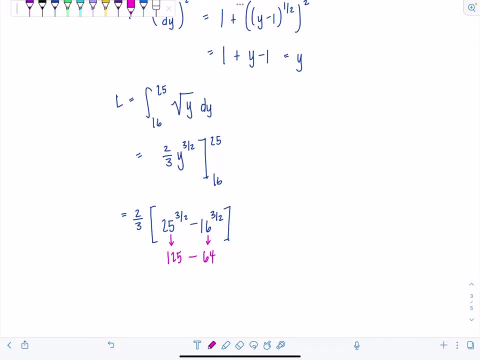 Oh beautiful. So 125 minus 64.. I'm going to take the square root of 64 to the three halves and then cube it, And then cube it. I want to take the square root of 64 and then cube it. 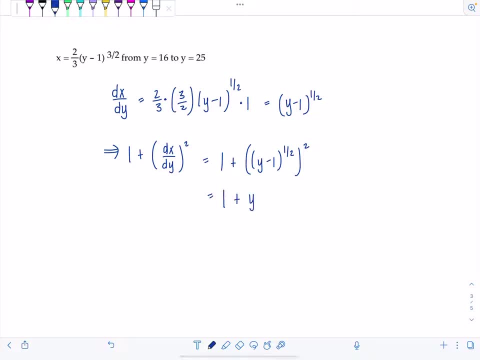 Oh, so let's integrate. Lovely, This is one plus y, minus one, which is just y. This is what dreams are made of. So arc length is going to be definite integral from 16 to 25. square root of y dy. 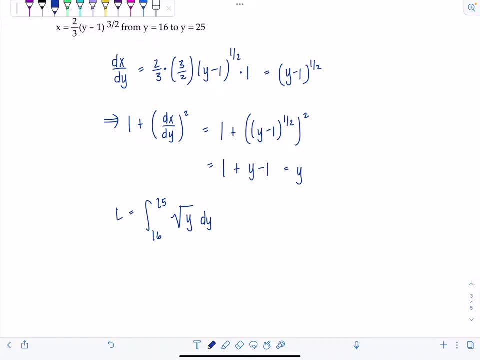 So square root of y, that's y to the one half. If I integrate I'm going to add one to the exponent, So it'll be y to the three halves divided by the new exponent, And then evaluate, And then I'm going to calculate this from 16 to 25.. 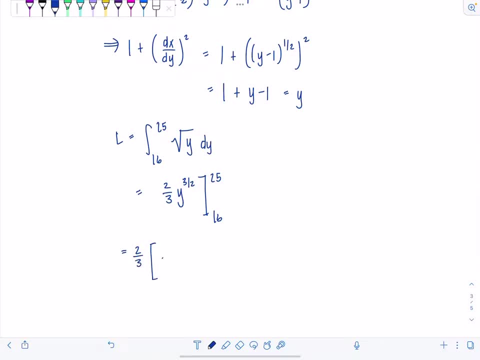 Okay. so we've got two thirds times 25 to the three halves minus 16 to the three halves. We don't need a calculator for this, Oh, no, no, no. So 25 to the three halves, you take the square root of 25 and then cube it. 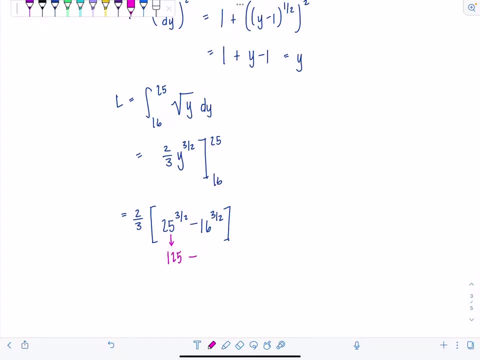 So five cubed is 125.. Same thing: 16 to the three halves. You take the square root, Because you have a two in the denominator four, and then cube it, That's 64.. Beautiful. So 125 minus 64.. 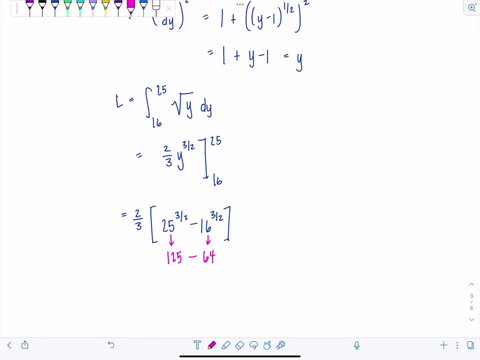 I want to say it's 61. Let me think, Yes, good, So this is going to be two thirds times 61, which is just 122 over three. All right, very nice, We doing okay. Last example, I think is a little clever, so I like doing it. 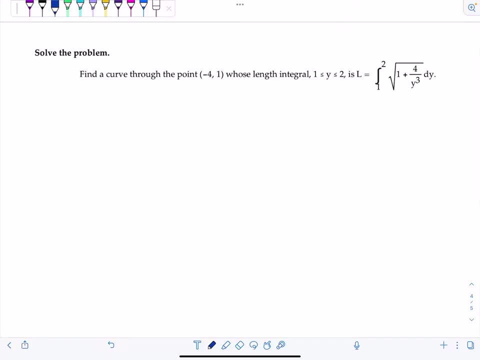 Find a curve through the point negative 4, 1, whose length integral from y equals 1 to 2, is given by the following: So they've already set up the formula for us to find the arc length. They want us to find the original curve, find the function. 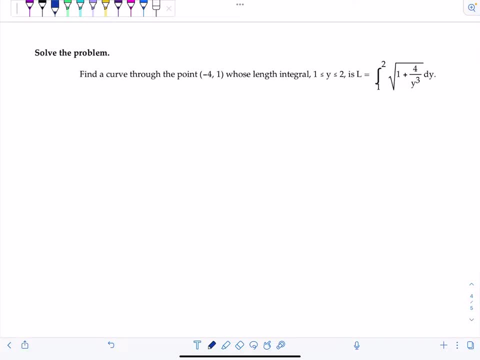 And I notice here we're integrating with respect to y, so probably we're going to find the original curve x as a function of y. Okay, Well, what do we know about this arc length formula If we're integrating with respect to y? this is c to d, right times, the square root of 1 plus dx, dy, squared dy. 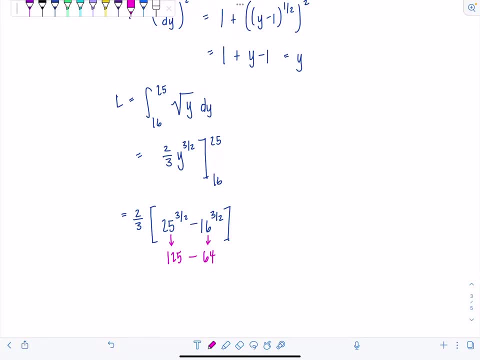 Beautiful. So 125 minus 64.. want to say it's 61. Let me think, Yes, good. So this is going to be 2 3rds times 61, which is just 122 over 3.. All right, very nice We doing okay. 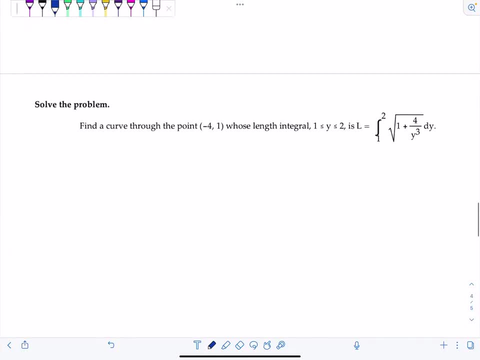 Last example I think is a little clever so I like doing it: Find a curve through the point negative 4: 1, whose length integral from y equals 1 to 2, is given by the following: So they've already set up the formula for us to find the arc length. They want us to find the original curve. 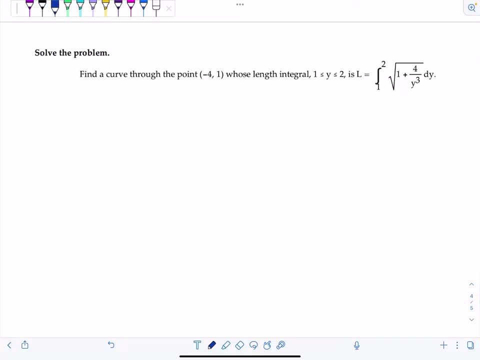 find the function, And I notice here we're integrating with respect to y, so probably we're going to find the original curve, x as a function of y. Okay, well, what do we know about this arc If we're integrating with respect to y? this is c to d right times, the square root of 1 plus. 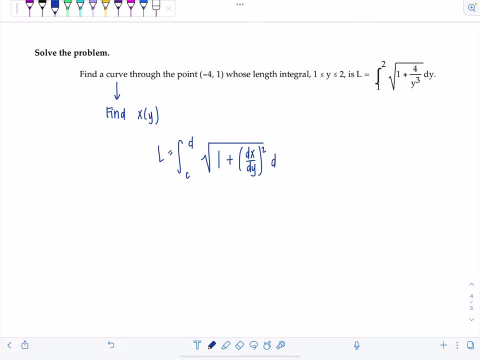 dx dy squared dy. So I'm trying to figure out what the function is x of y. I have its derivative squared. Maybe that's going to help me. So let's look here. dx dy squared is equal to: instead of 4 over y cubed, I'm going to write it as 4y to the negative. third: 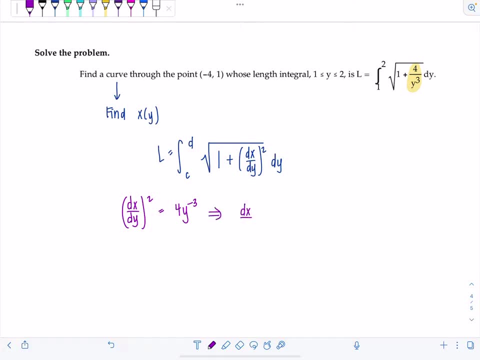 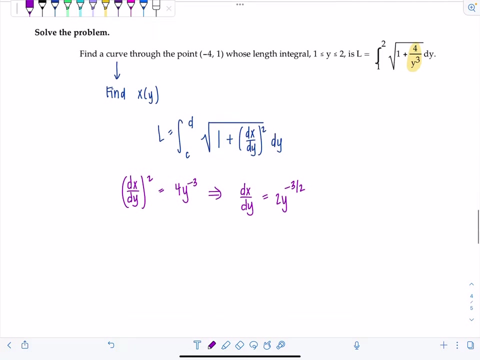 And then if I take the square root of both sides, that means dx dy is equal to 2y to the negative three halves. I didn't put plus or minus because, notice, the limits are from 1 to 2, so nothing's going to be negative. All right, this is basically a differential equation, right, I can? 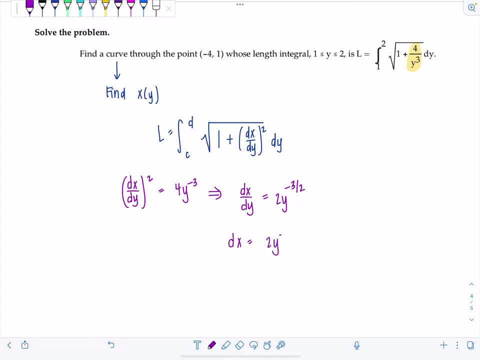 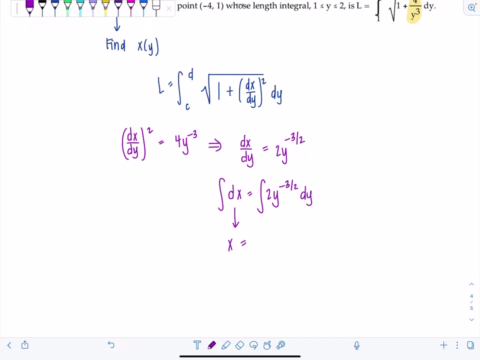 move the dy over to the other side. So dx equals 2y to the negative three halves dy, And then I can integrate both sides And we're going to have x equals. if I integrate y to the negative three halves, I'm going to add 1 to the exponent, So it would be y to the negative one half and divide by: 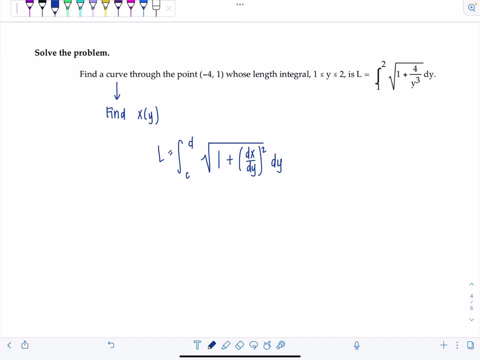 So I'm trying to figure out what the function is. So if I take this x of y, I have its derivative squared. Maybe that's going to help me. So let's look here. dx dy squared is equal to: instead of 4 over y cubed, I'm going to write it as 4y to the negative. third. 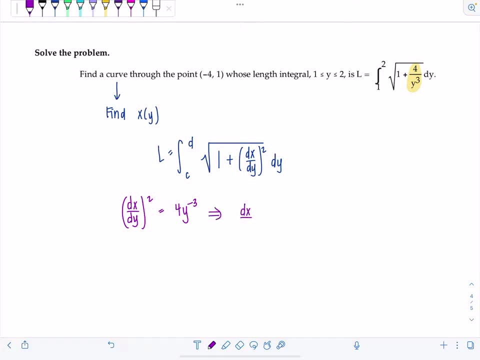 And then if I take the square root of both sides, that means dx dy is equal to 2y to the negative three halves. Okay, I didn't put plus or minus because, notice, the limits are from 1 to 2, so nothing's going to be negative. 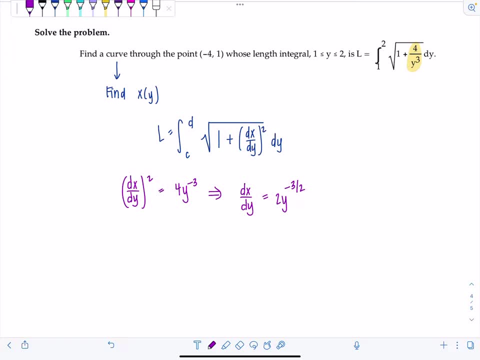 All right, This is basically a differential equation, right? I can move the dy over to the other side, So dx equals 2y to the negative three halves dy, And then I can integrate both sides And we're going to have x equals. 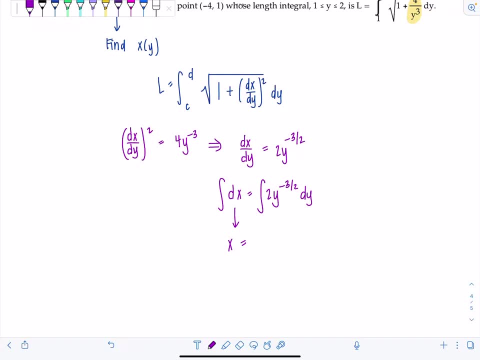 Okay, So we're going to have x equals 2y to the negative three halves dy. So if I integrate y to the negative three halves, I'm going to add 1 to the exponent, So it would be y to the negative one half and divide by that exponent. 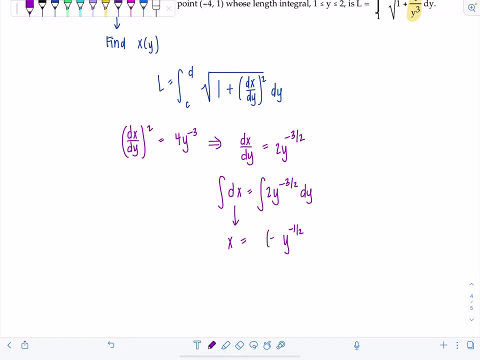 So I would divide by negative one half. That's the same as multiplying by negative 2. And I already have a 2 in the front, And then plus c. So I can see right now: x is equal to negative 4y, to the negative one half plus c. 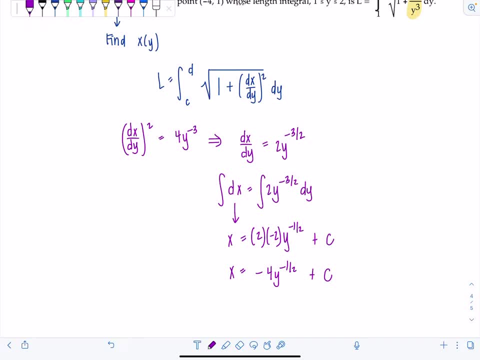 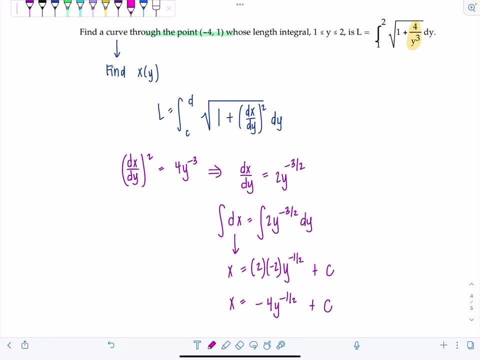 Good, How can I find c? Well, they gave me a little extra info I haven't used. yet It told me that the curve goes through the point 4, negative 1.. So I'm going to substitute in negative 4 for x and 1 for y and find c. 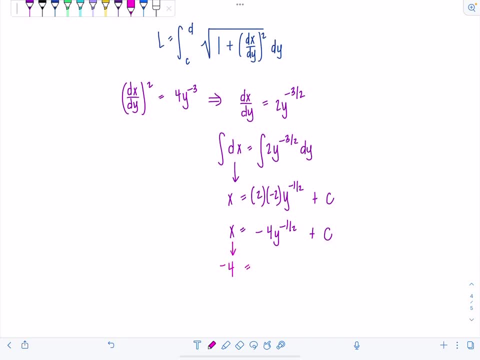 So x is negative 4.. y was 1.. And then I can see: if I add 4 to both sides, c is just 0.. Oh, Okay, So then we have x equals negative 4y to the negative one half.